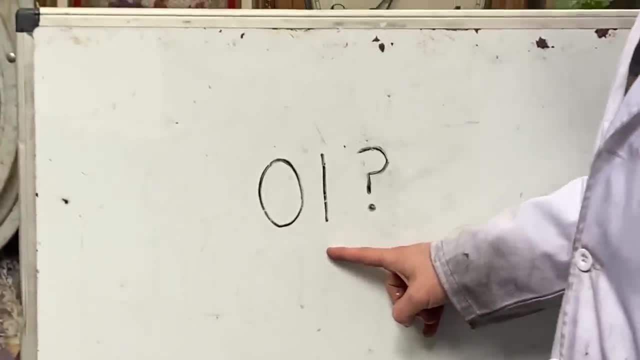 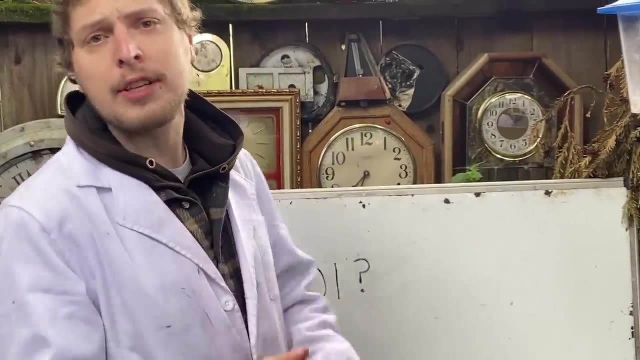 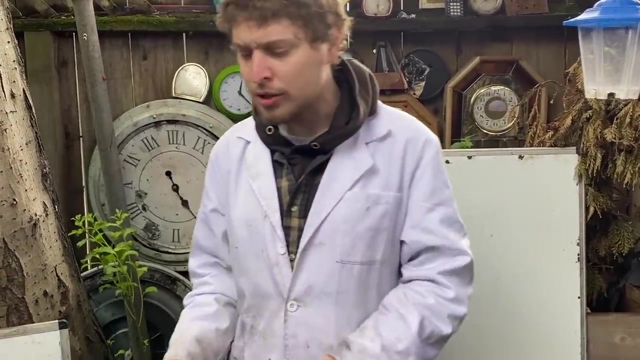 the digits zero, one and a third digit that isn't two. Now we can actually jump into why and how this balanced ternary might work as an alternative to binary by imagining some puzzles where we're trying to weigh some items. Let's say I have an. 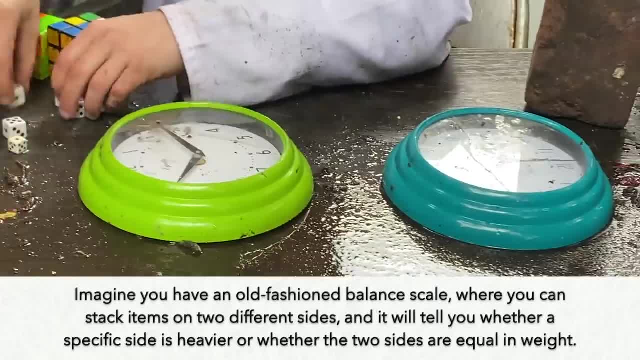 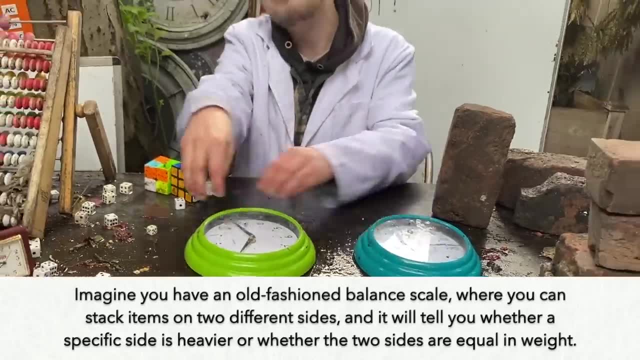 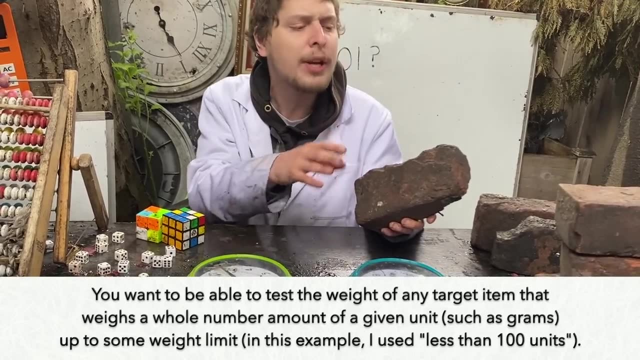 old-fashioned balance scale that'll just tell me whether the two sides are equal in weight or whether one side weighs more than the other. And I want to be able to test the weight of any item that weighs a whole number, amount of some unit of weight up to some given size. 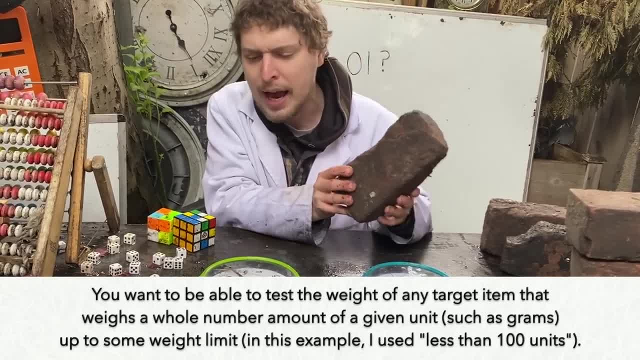 Let's say I have a number that weighs a whole number amount of some unit of weight. up to some. Let's say I have a number that weighs a whole number amount of some unit of weight. up to some, Let's say it weighs less than 100 of that unit. What would be the ideal collection of weights for? 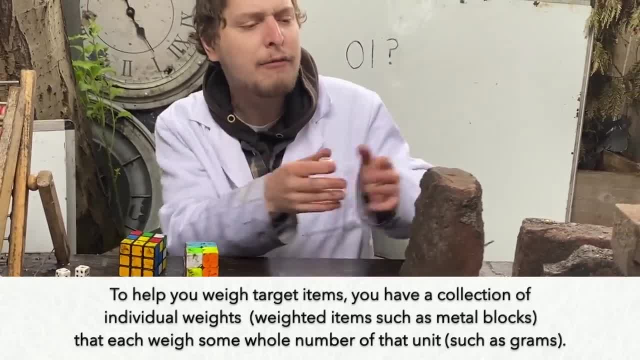 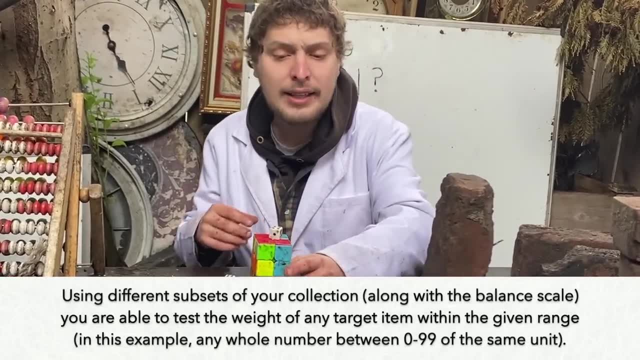 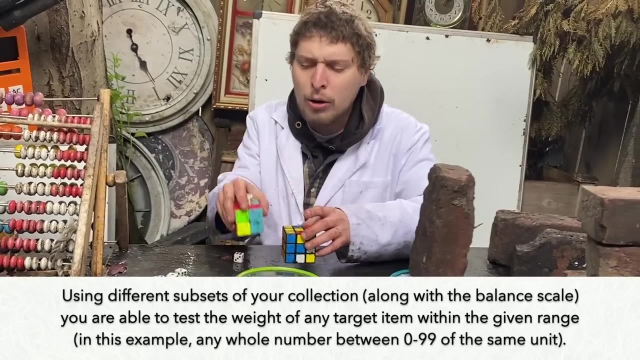 me to have. that would let me test any of those weights. Well, my collection of weights would need to have some subset of it that let me calculate each and any possible whole number, weight between zero and 99 in this case. But let's say I also wanted my set of weights to have the minimal amount. 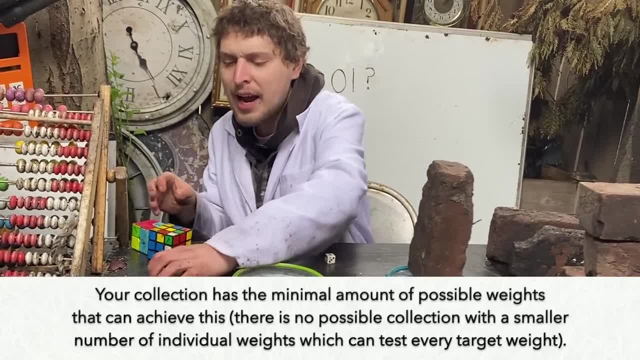 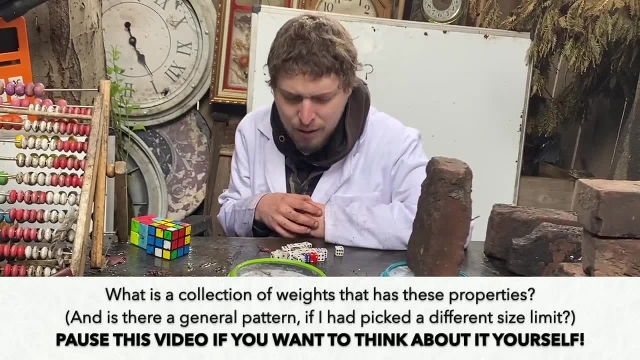 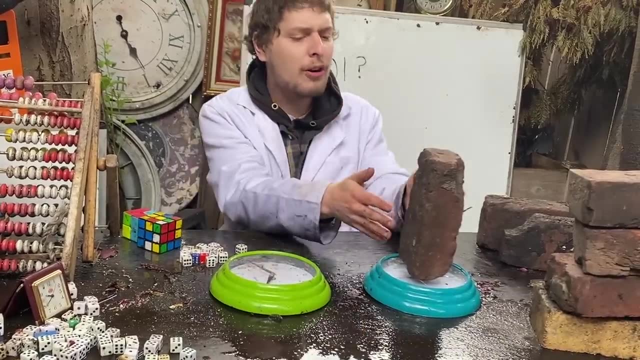 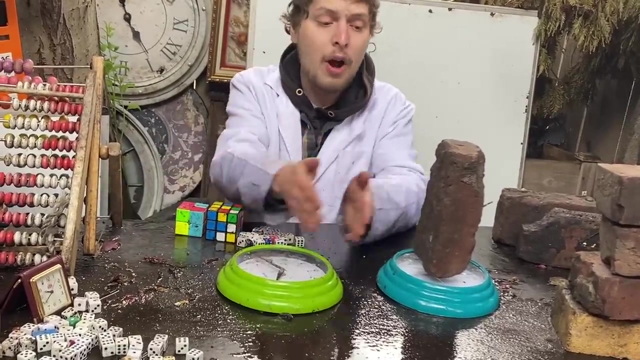 of total weights in it, so that I didn't just have like 99 one unit weights and used somewhere from zero to 99 of those. Well, if you first encounter that problem, you probably assume that my target weight is on this side and the weights in my collection are either being unused or put on the 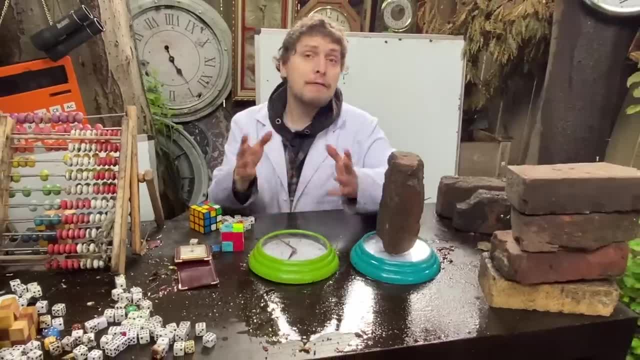 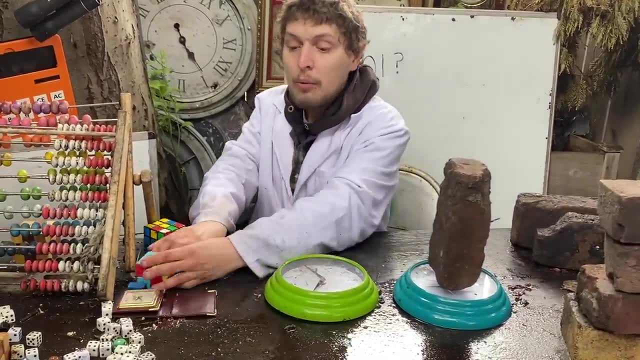 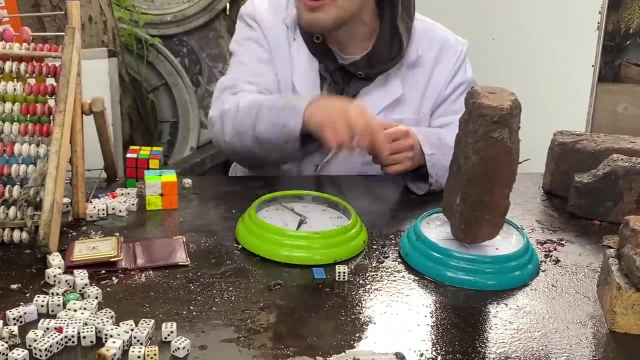 opposite side of the balance scale. And if that is the setup, and that's what we're allowed to do, then my ideal set of weights would have one that was one unit, one that weighed. let's say, this one is two units, something that weighed four units. 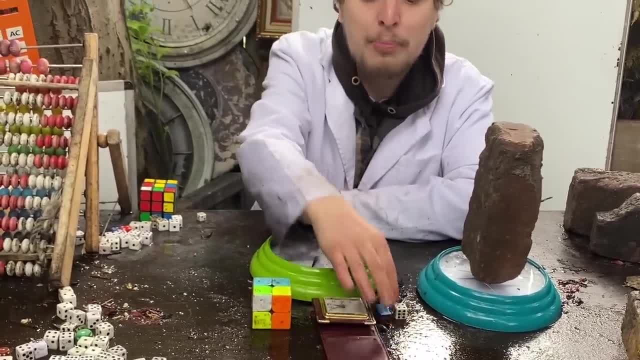 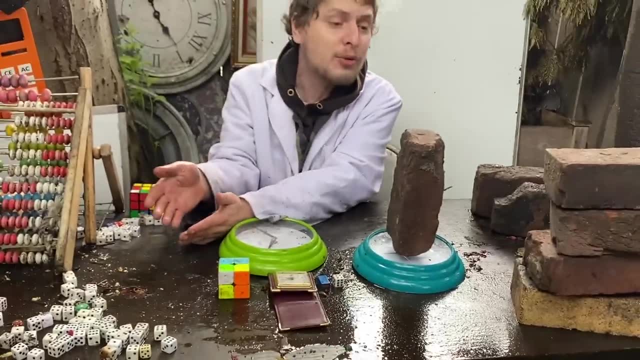 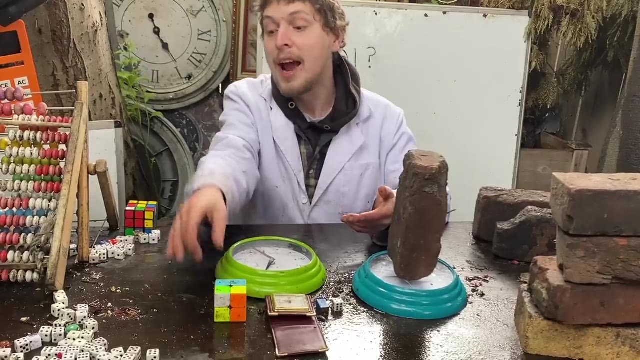 something that weighed eight units and all of the powers of two, including two to the zeroth power, which is one up through the biggest one before our target weight. In this case, we would also include a 16 unit weight, a 32 and a 64. And that fact that we can 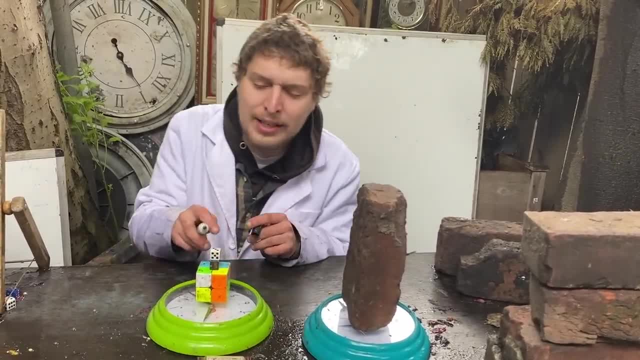 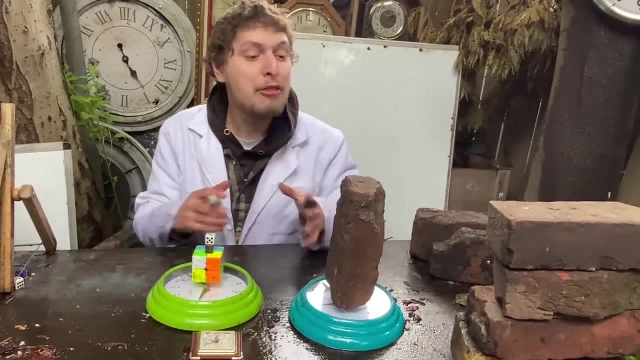 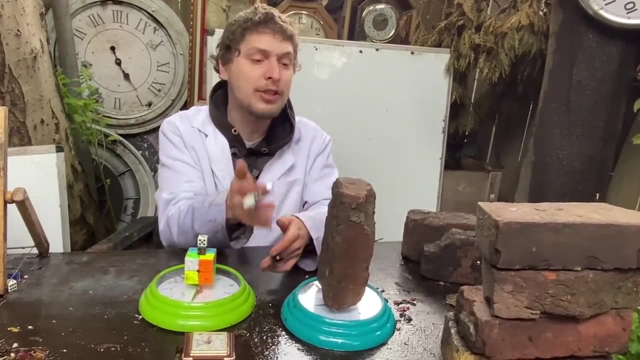 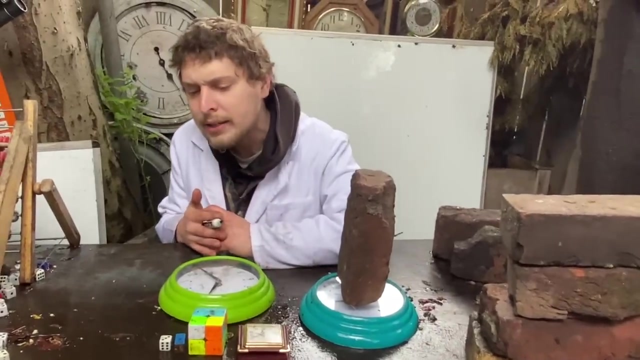 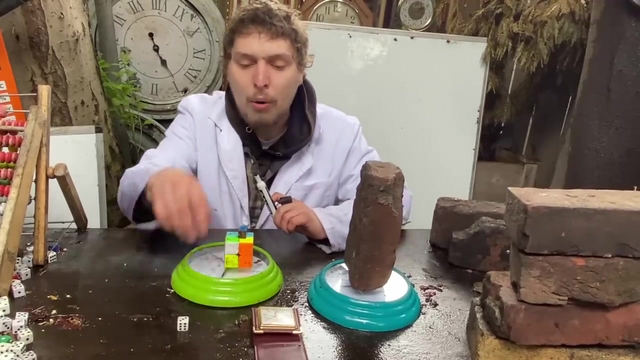 take some subset of the powers of two and add them up to any non-negative integer is actually the same fact that the base of binary or base two can represent any of those numbers that the weights were using, just the digits 0 and 1.. Any of the target weights could be made from using 1 of some of them and 0 of. 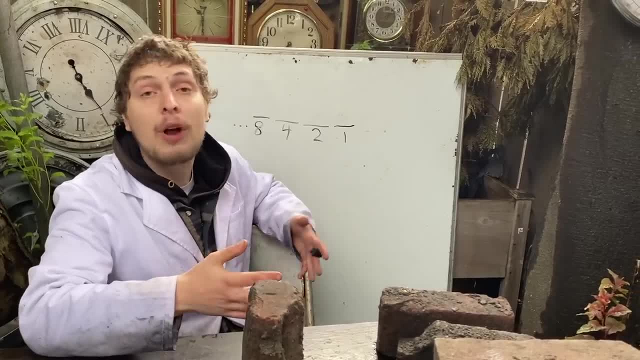 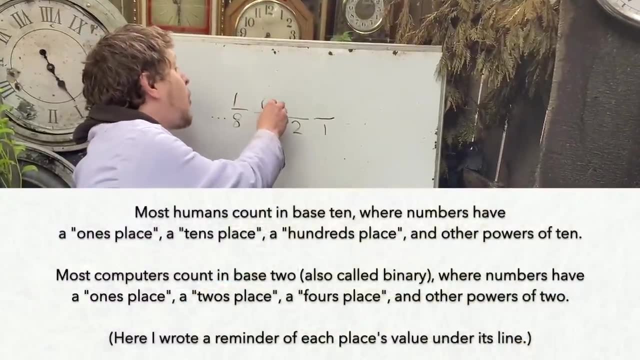 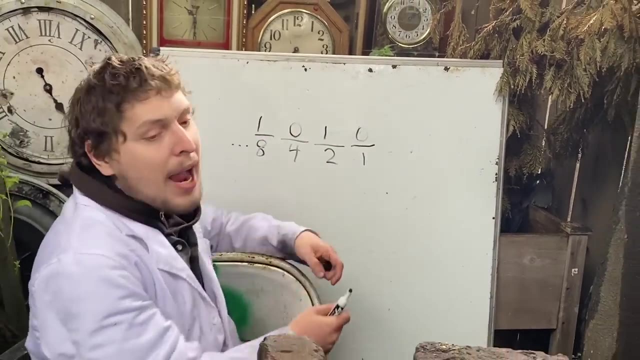 some of the others. For example, if I wanted to write 10 of a thing in binary, I would use 1,, 8, no 4s, 1, 2, no 1s, and that 8 and 2 add up to my 10.. Just like if I need to weigh something that. 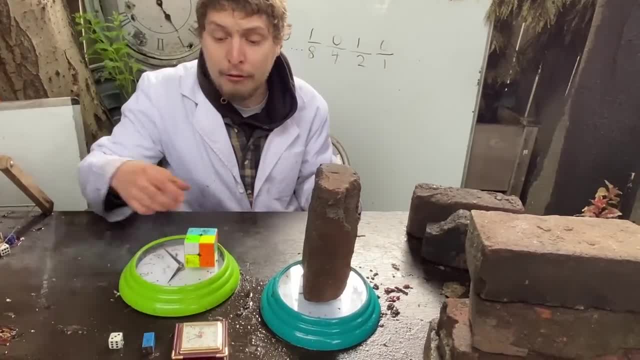 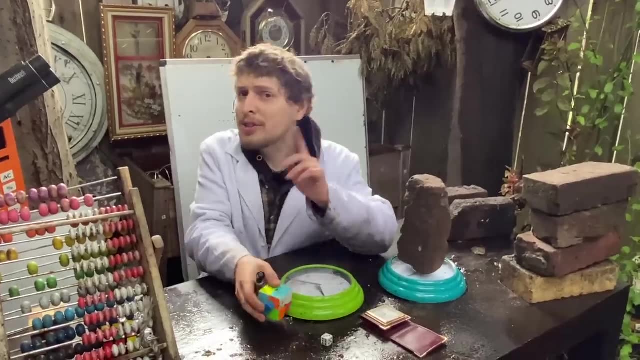 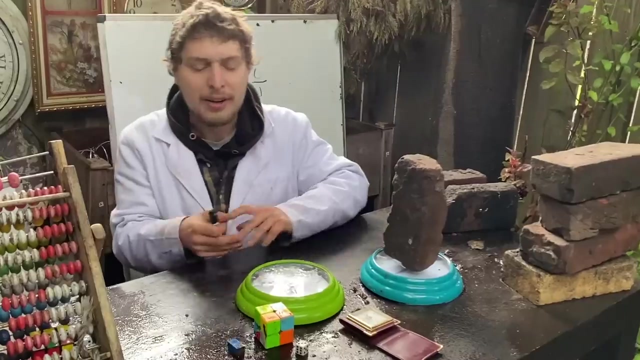 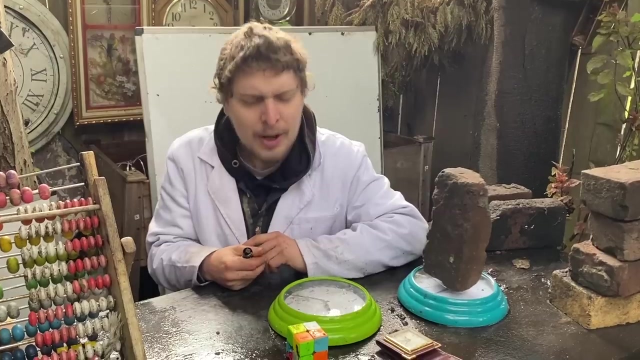 weighs 10 units. I can use 1 of my 8-unit weights and 1 of my 2-unit weights, But here's the thing: The powers of 2 aren't actually the answer to the original question. They're not the ideal set of weights that would let me calculate any target weight, Because I 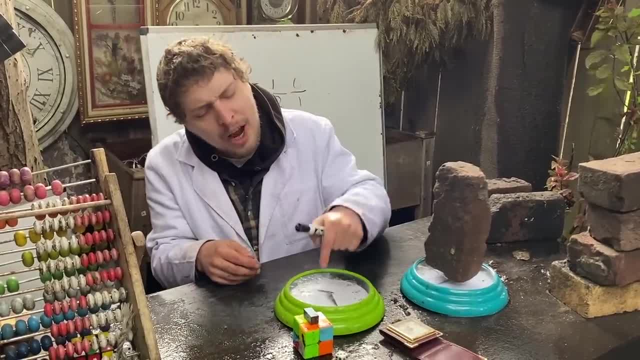 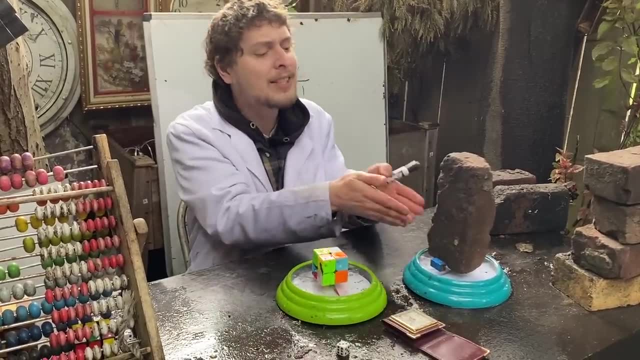 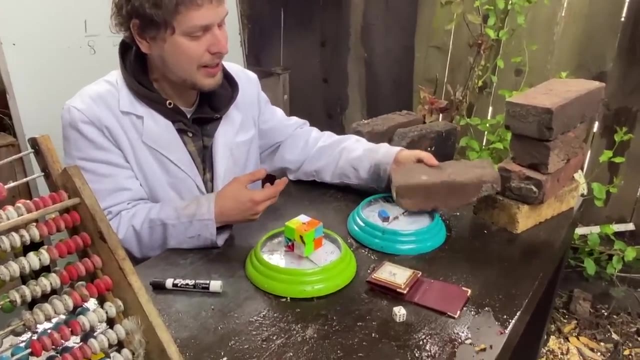 don't have to put weights from my collection just on the opposite side of the target. I could put weights from my collection on that same side too. Like if, for example, this brick weighed 6 units, then pretend the balance scale still weighs 6 units. 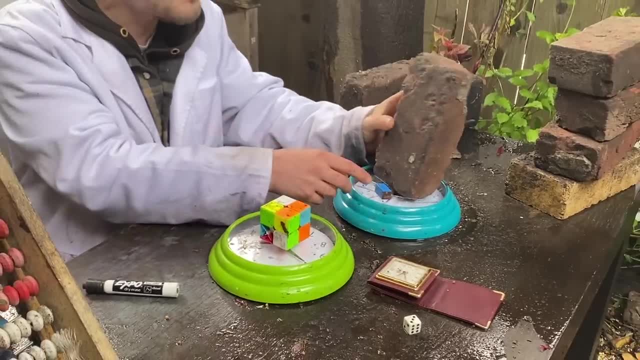 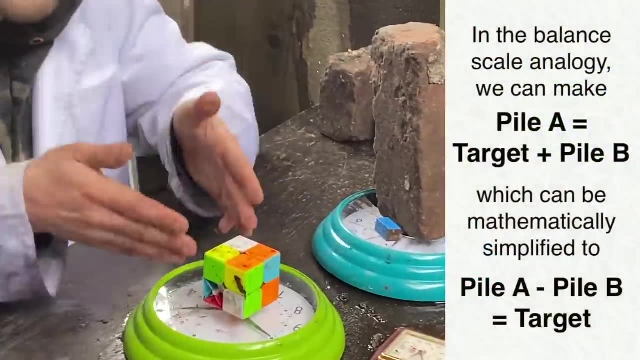 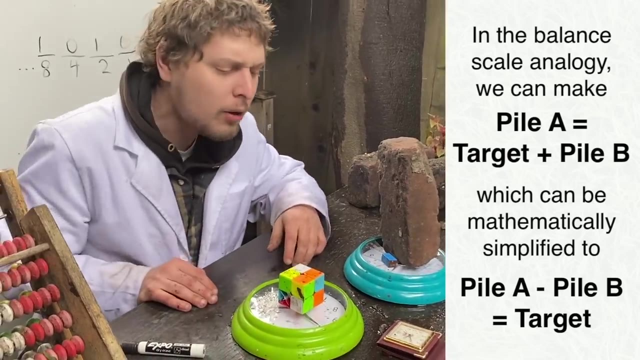 It works in our analogy. Then having a 2-unit weight here and an 8-unit weight there would confirm its weight in the same way that 8 minus 2 is 6. So knowing that we can stack our weights on either balance scale and the ones here help add toward a target weight. 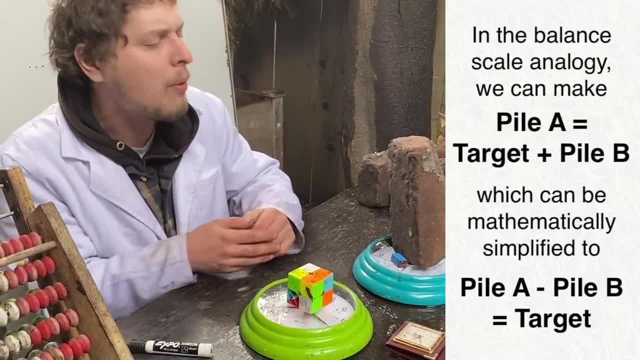 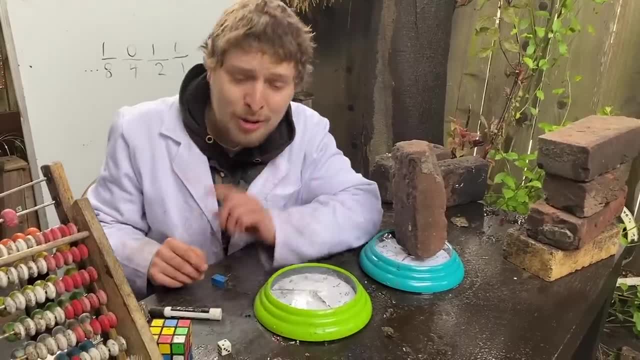 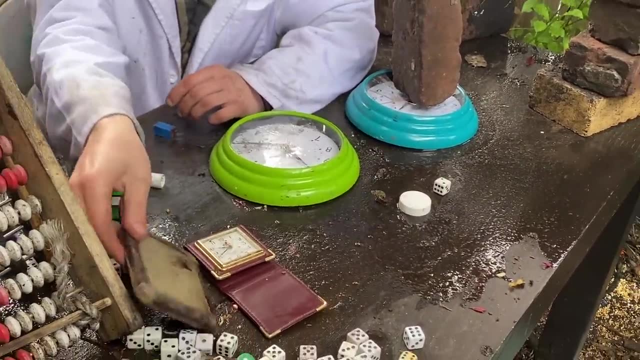 while the ones here subtract in a way. what would the ideal or minimal set of weights for our collection be? My ideal collection would include a 1-unit weight, a 3-unit weight, a 9-unit weight, a 27-unit weight. 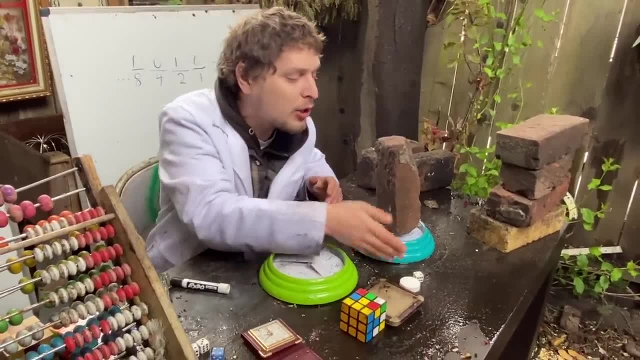 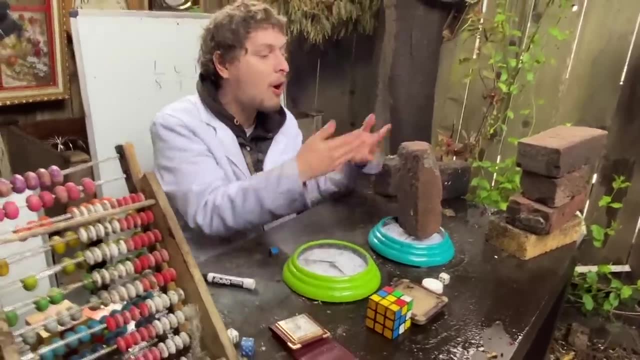 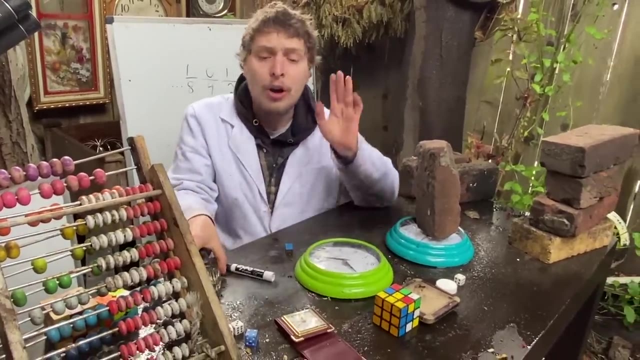 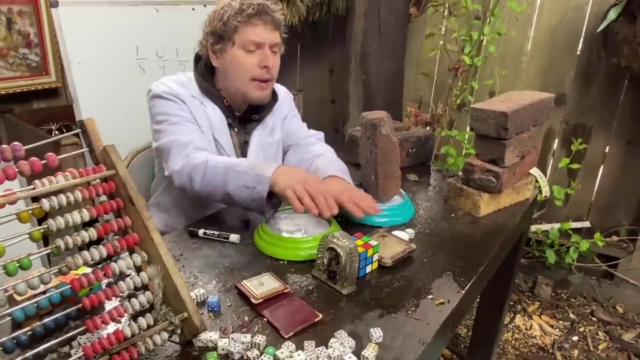 and all of the powers of 3, including the 0th power, 1,, up to whatever power of 3 was before our target amount. In the case of it weighing a whole number, up to 99,, we would also need one weighing 81,, the next power of 3.. And there's some way of assembling. 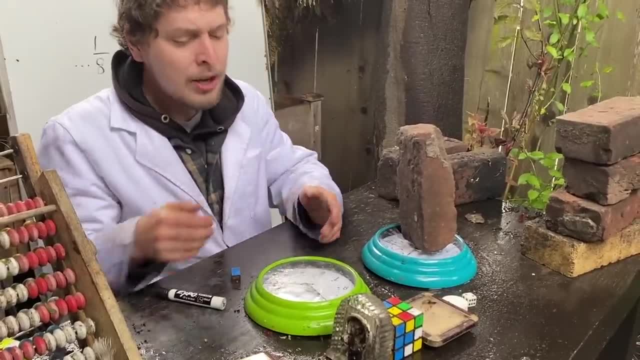 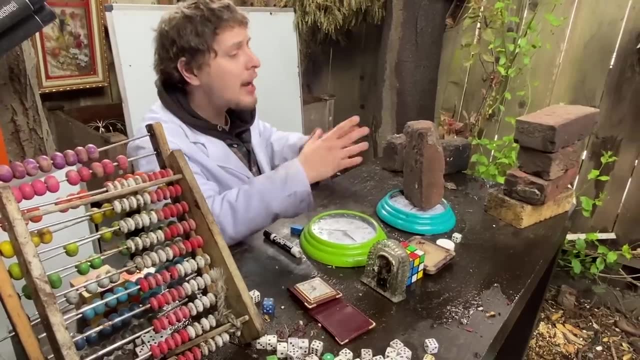 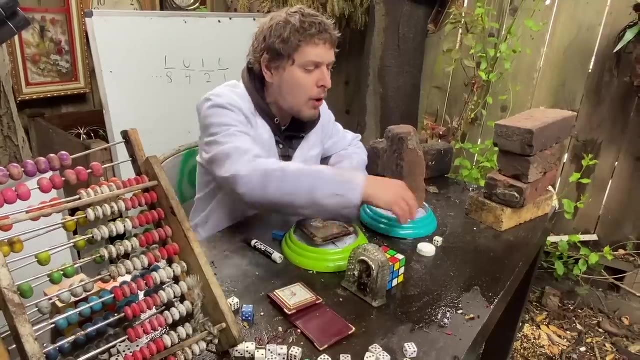 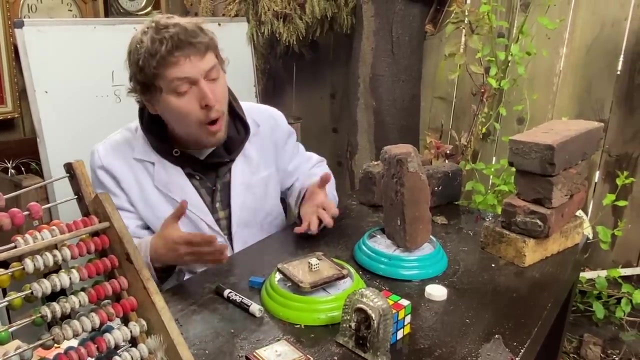 these in different combinations to add and subtract toward any of those target numbers. For example, if I needed to calculate something that was 10 worth of weight, I could use my 9-unit weight, whereas if I needed to calculate something that was a weight of 20, it would be a little trickier. 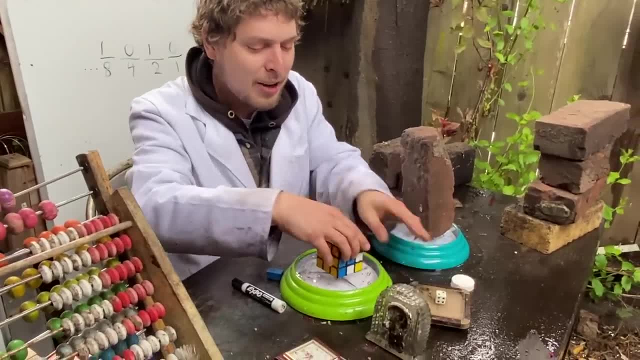 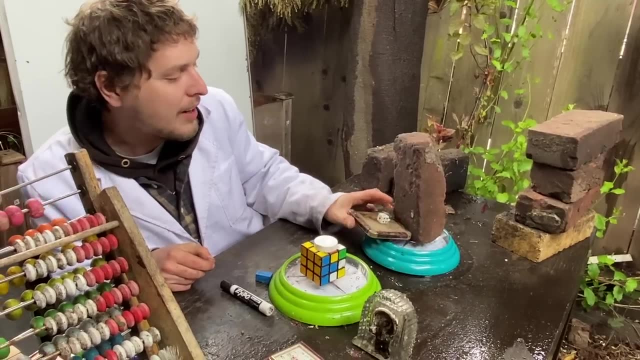 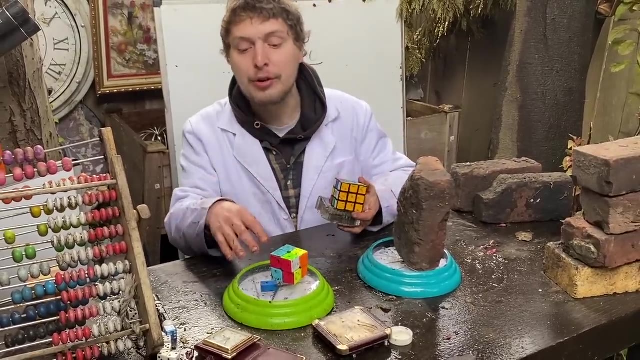 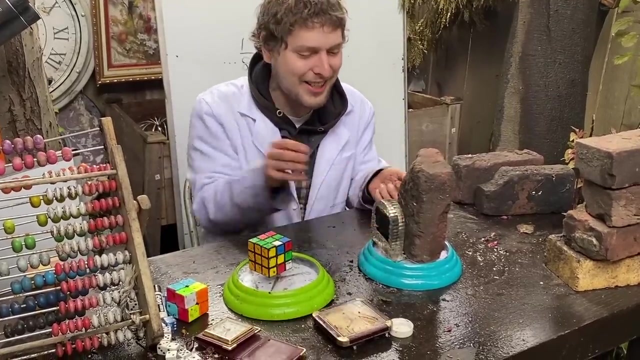 but I could still do it. I would need to take 27 there plus three more there and then put nine and one on the side of the target. so if the situation where we have the powers of two just on this side is like binary, is there a base that this new situation is like? 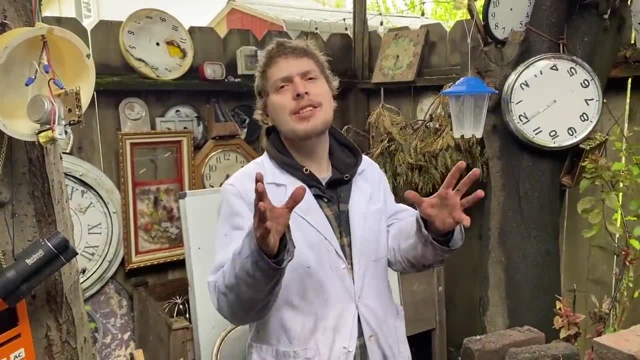 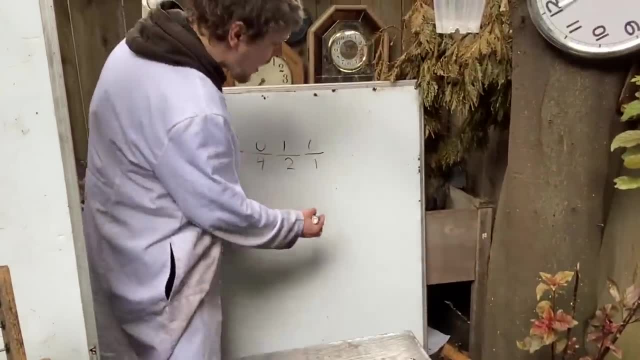 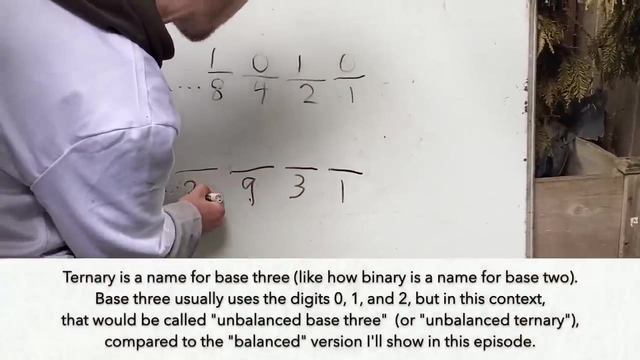 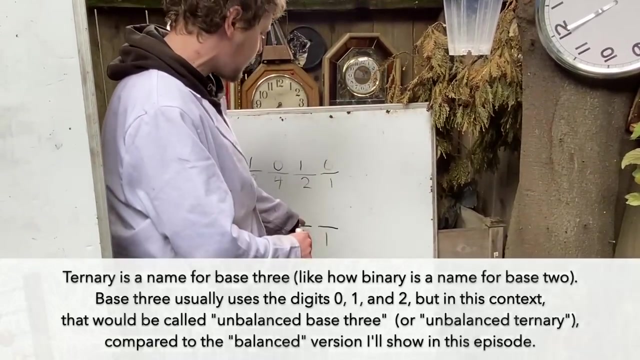 there is, and that base is called balanced ternary, with the powers of three. as our collection of weights, that's like having spots in a number that are worth powers of three. except in normal base, three or ternary, we'd be using zero, you one or two of each of these, and in this case 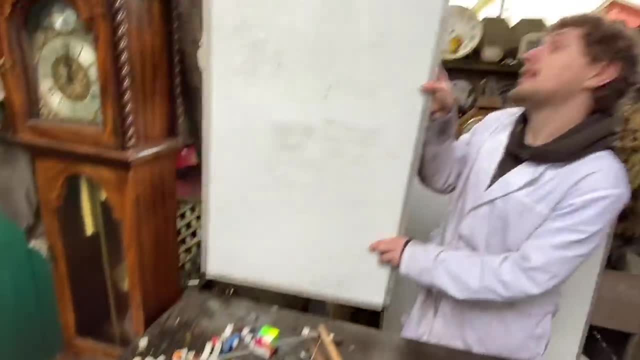 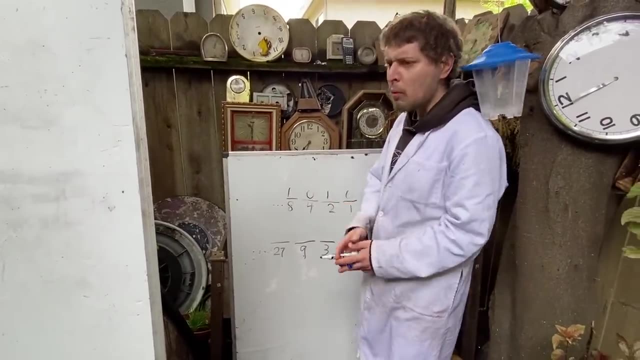 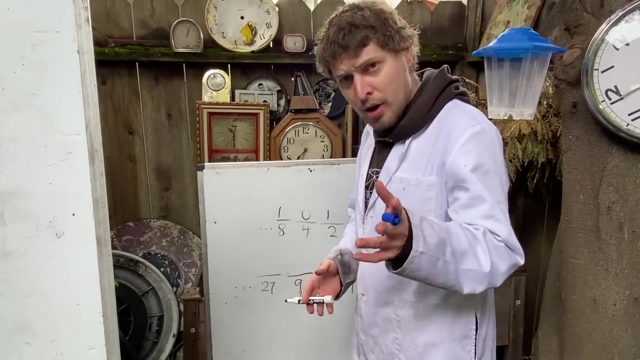 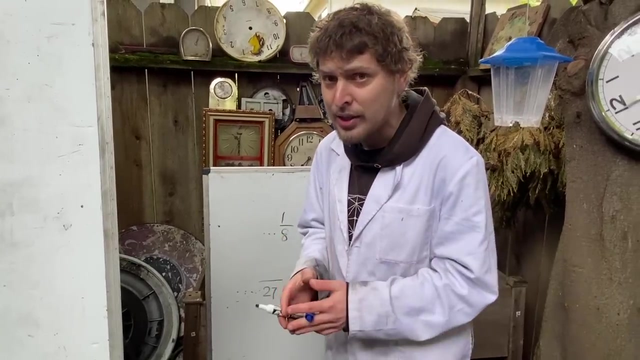 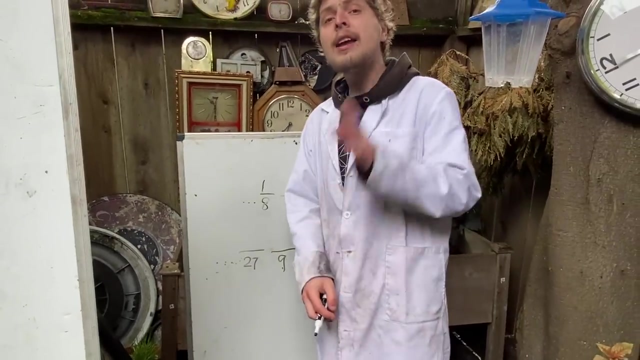 in this case, we had none one, or removing one as an option, which is like zero one and negative one as our possibilities now, unlike my older episode about counting in negative bases- yeah, the negative, the negative and the number that each place represented were powers of a negative number- here the negative comes in. 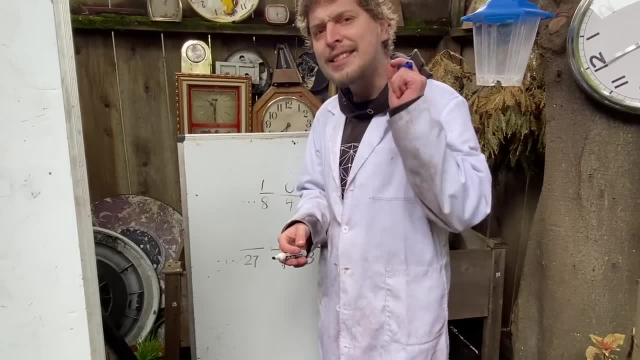 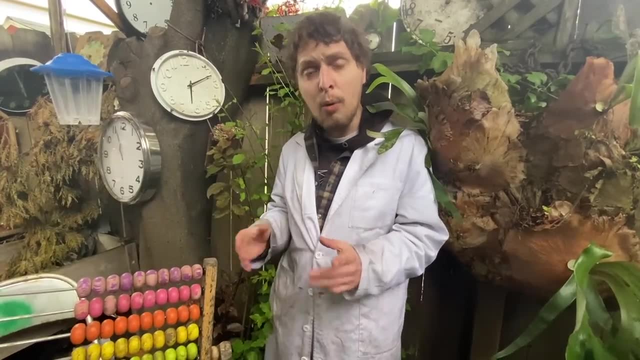 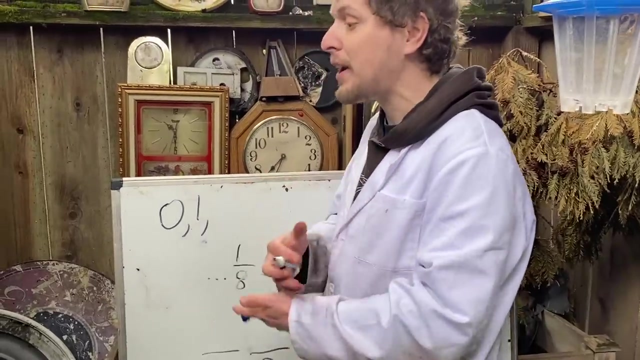 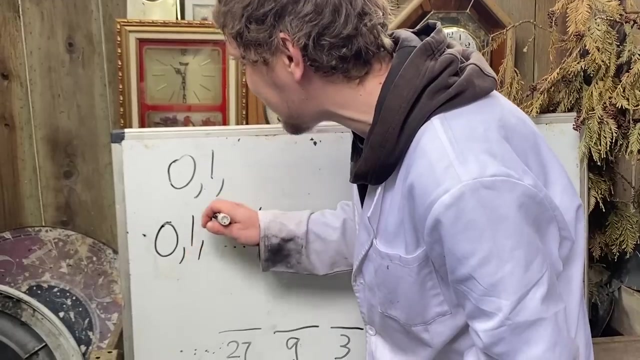 as one of the options for what a digit can be In balanced ternary. the three digits you use represent zero one and negative one. Now, there's not really a standardized third symbol that everyone uses when talking about balanced ternary. Some texts write zero one and t for the negative. 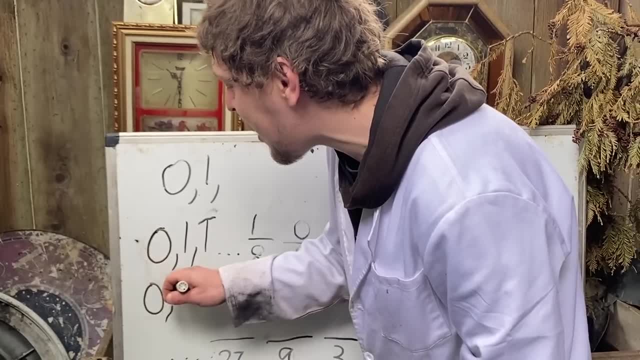 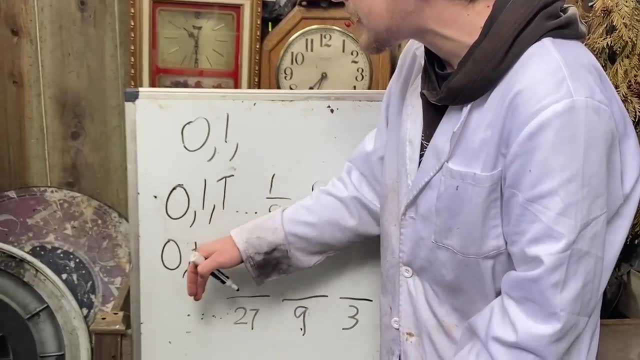 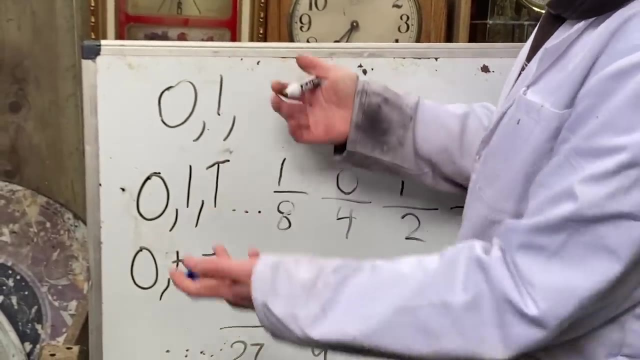 one. Some write zero, plus to represent one and minus to represent negative one, which sort of hints at how they have the same magnitude, just different signs or directions. they're taking it And what we'll do, sort of a mix of those two. 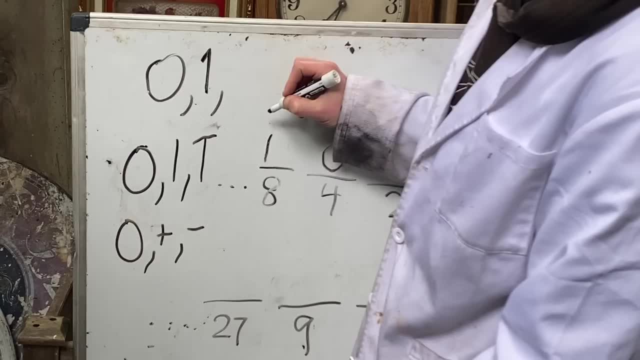 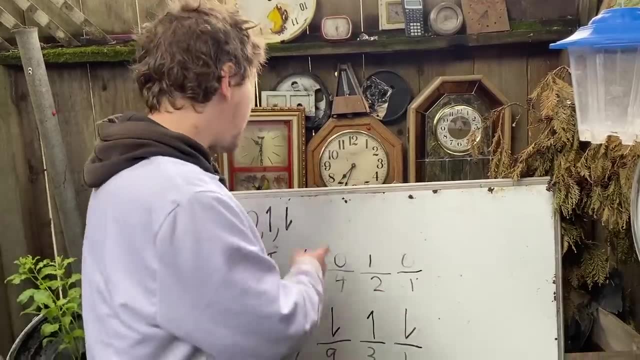 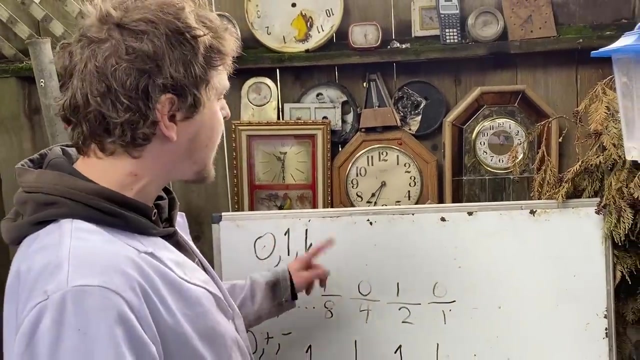 is just making a. this one have a crook on top of it, so we can write an upside down one to represent negative one. I also chose to have arrow-like symbols for these because it hints at how computers could actually encode these three states. In a more typical binary computer, this structure of zeros and ones is made. 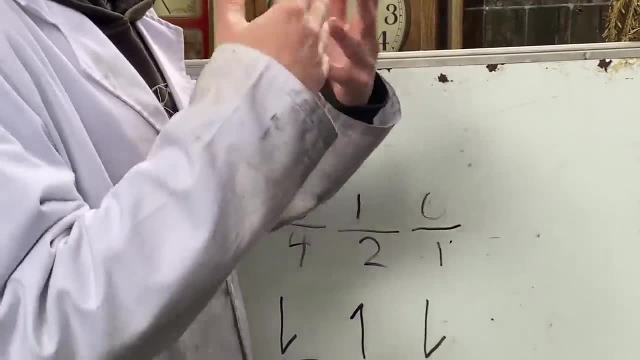 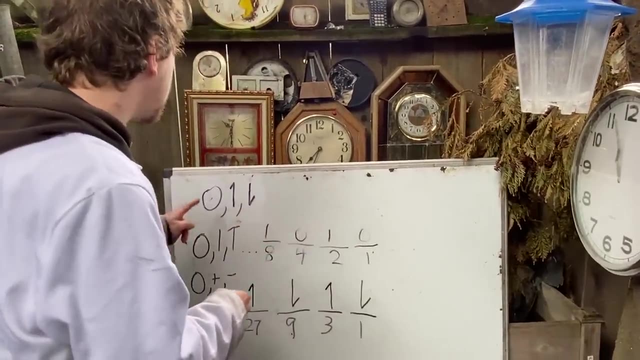 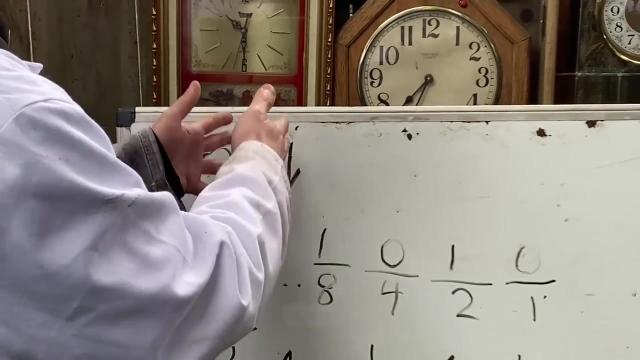 from the computer having little parts that are either in an off state, signifying a zero, or an on state, signifying a 1. And here we still have an off state and now sort of have two types or directions: the on state could be in: 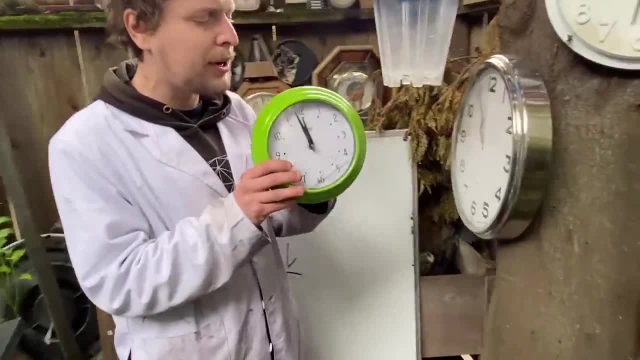 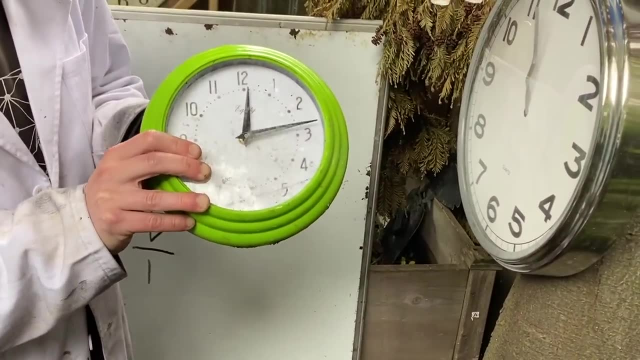 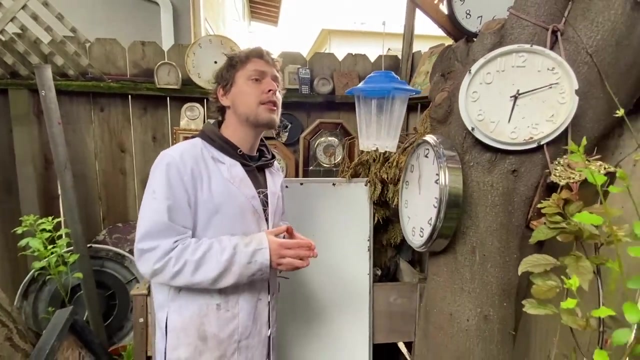 Like if our computer could have a part putting out an electrical charge, either clockwise through something, counter-clockwise through something, or not at all, Or if it was receiving light. either hor Setting off a signal or using关's signal is done using a straight line, kind of striking out the elements. 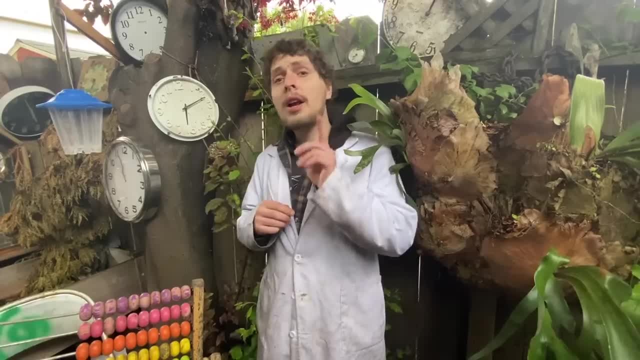 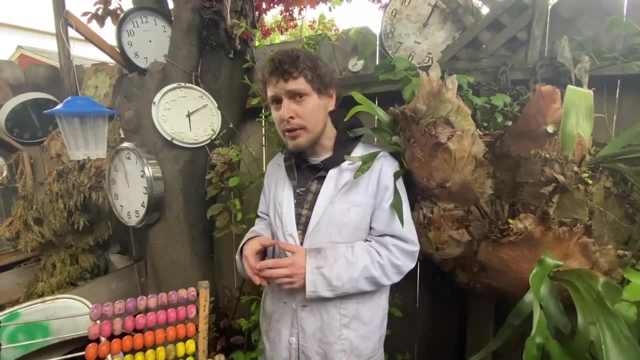 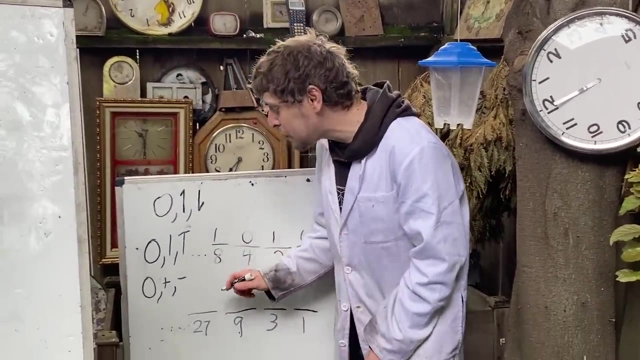 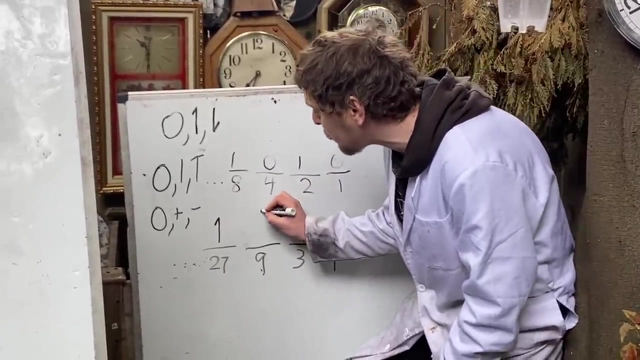 horizontally, vertically or not at all. Now, knowing that a computer could encode those three states, how do you turn them into specific numbers like binary? can Remember how I said: to make 20 using those weights, We would have used 127,, 13, and then we would have removed one of the nines. 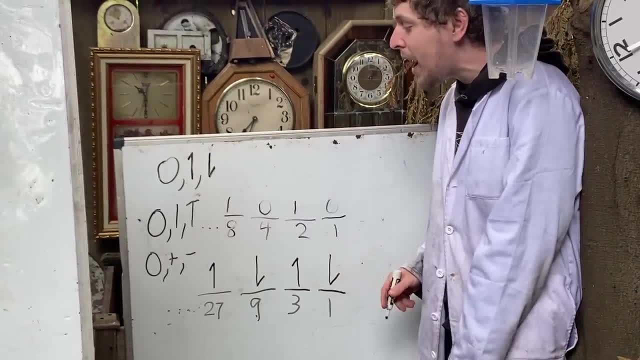 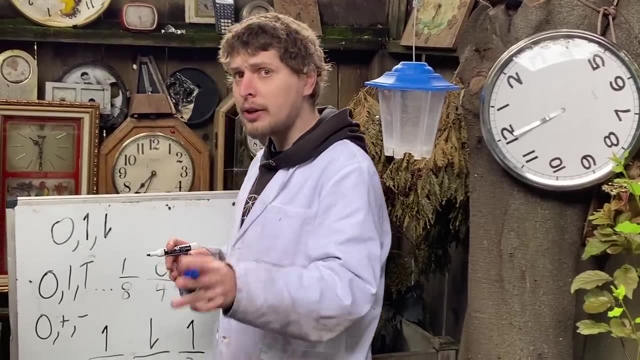 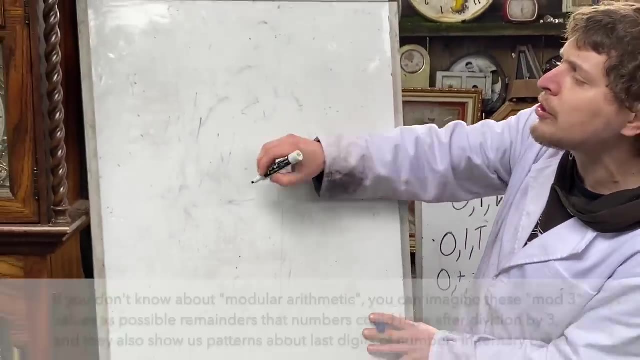 and one of the ones. Well, this would be a way balanced ternary could express the number 20.. And for those who remember how I've shown in earlier episodes how the last digit of a number in a given base is similar to the patterns of modular arithmetic, where we imagine a clock, 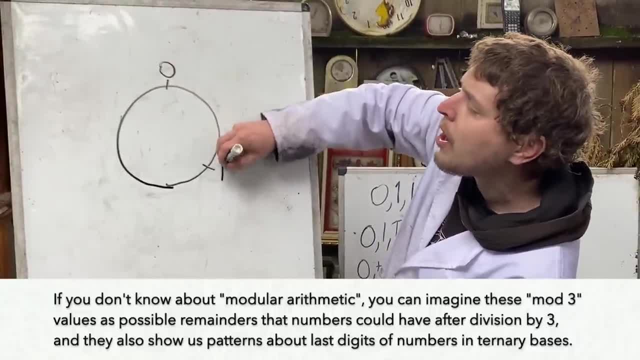 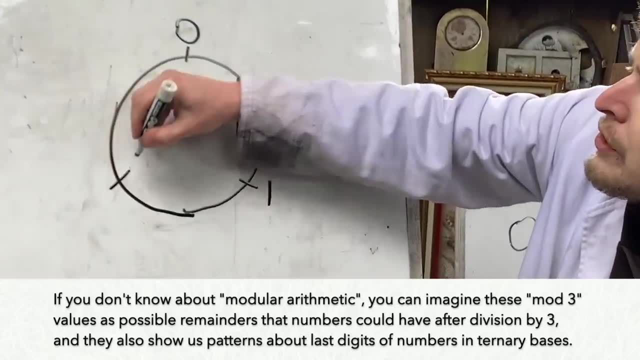 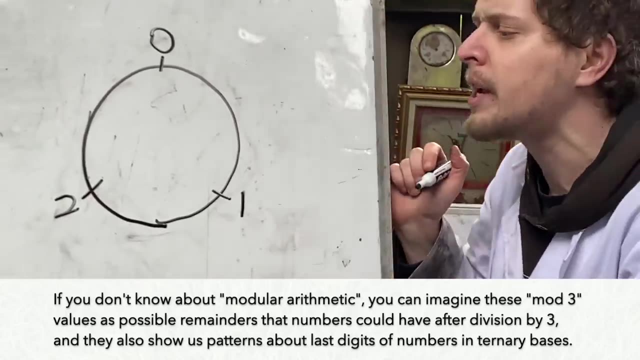 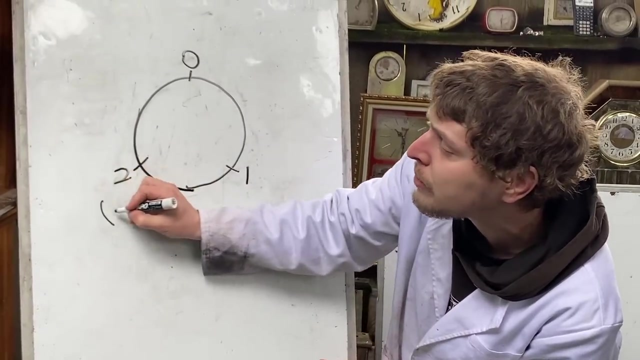 ranging from zero to one less than the base number, And typically in base three we would have zero, one and two, which is the typical way we've analyzed mod three, but we can call the values congruent to two in mod three the values congruent to negative one. 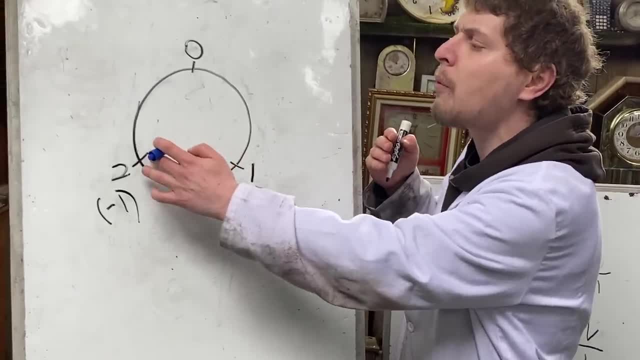 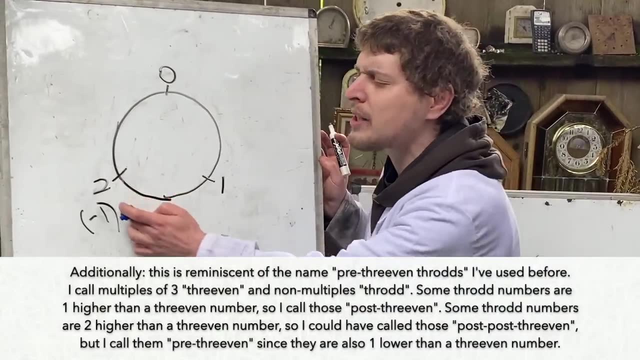 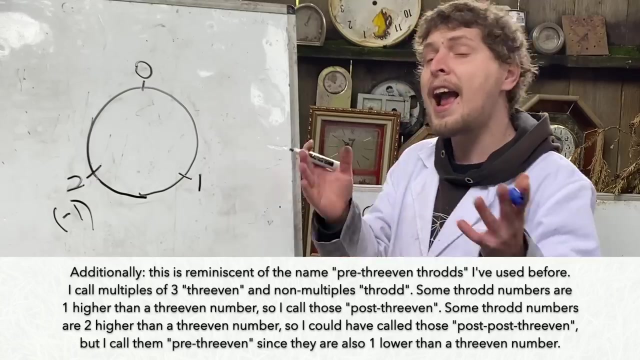 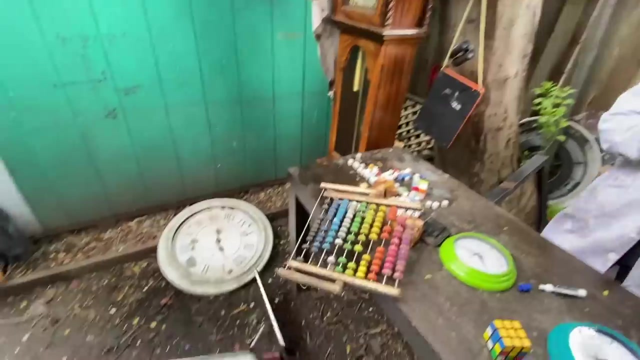 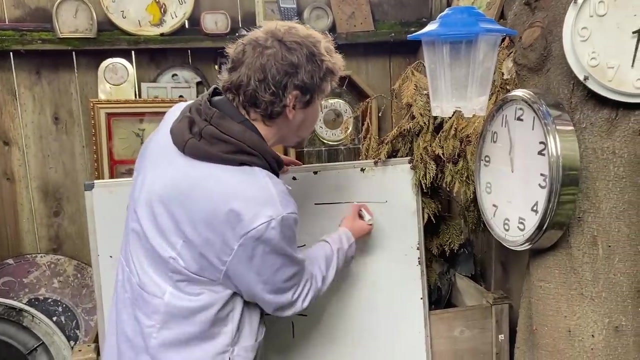 in that mod as well, because this is sort of one hour before the start, And so in mod three both of these languages exist. captures the patterns of both the normal ternary and the balanced ternary. Now, balanced ternary isn't the only possible balanced base Beyond balanced ternary, which used 0,, 1, and a symbol. 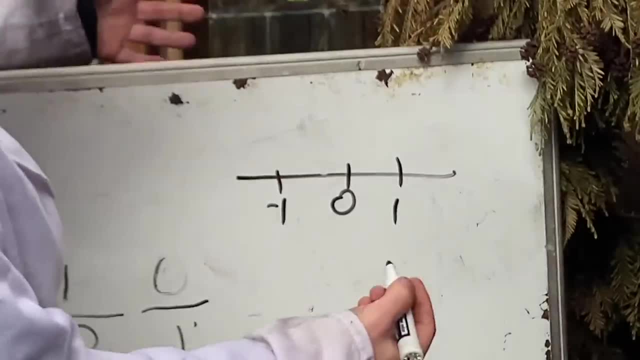 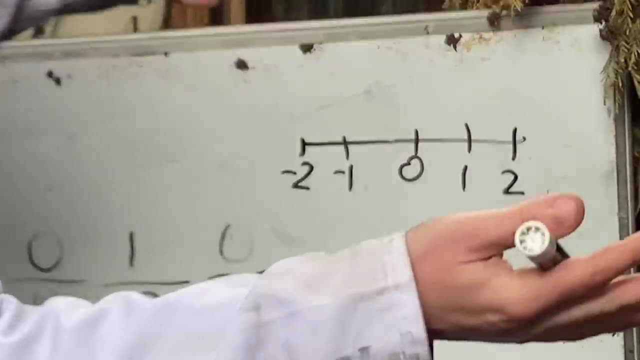 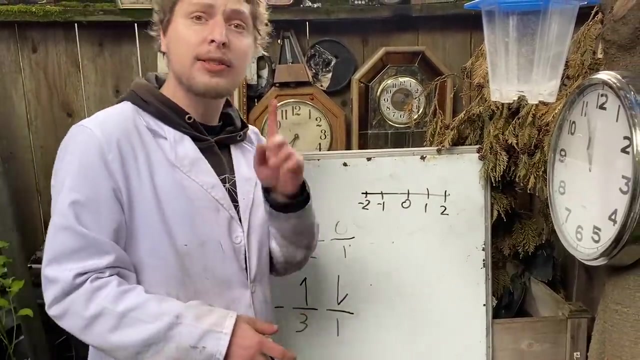 for negative 1,. we also could make balanced base 5 using 2 and negative 2, or balanced base 7, or any odd number. These balanced bases have a nice symmetry that typical bases don't and that actually gives them some mathematical superpowers, which I want to show you using the 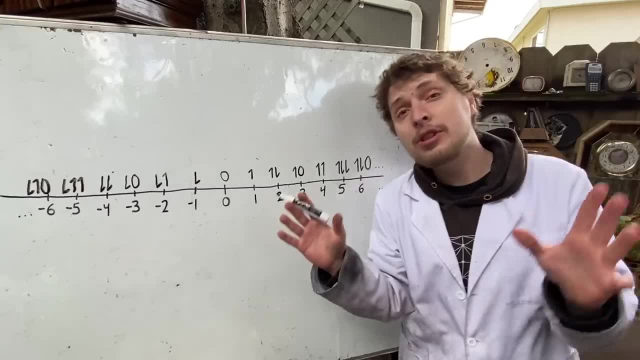 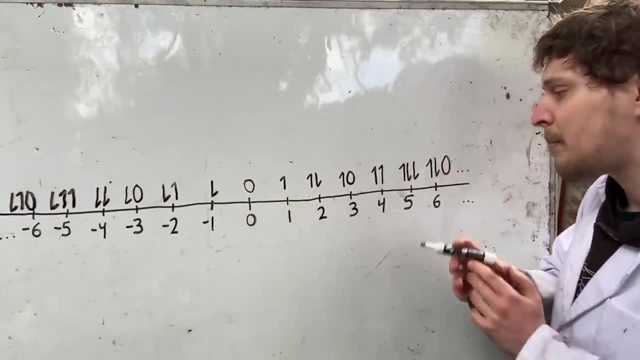 simplest of them, balanced ternary. Here's a stretch of number line with how we can use the number line to calculate the number line. Here's a stretch of number line with how we can use the number line to calculate the number line. We know numbers written on the bottom and how balanced ternary could write them on top. 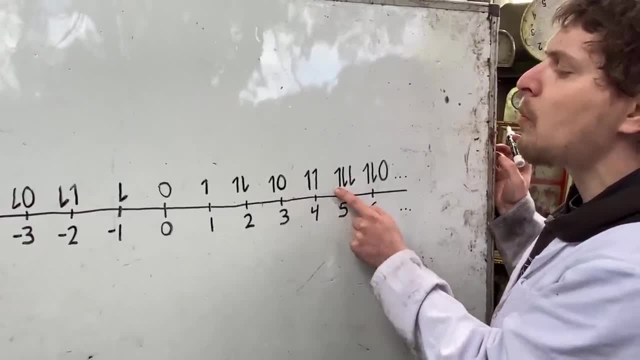 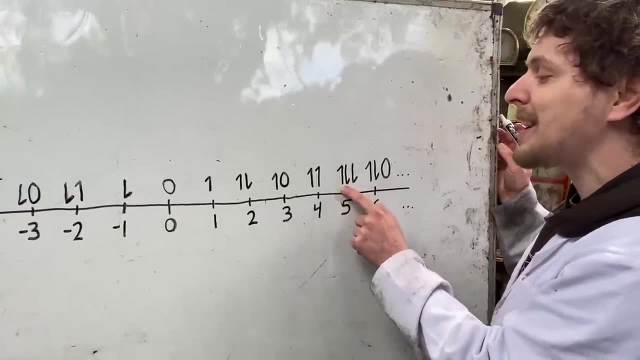 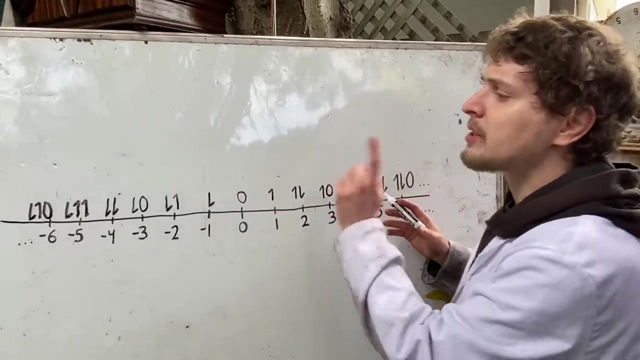 like the number 5 can be written with 1 of the 3 squared's place, which is 9's negative 1 of the 3's place and negative 1 of the 1's place. One cool trait about these balanced bases is how they 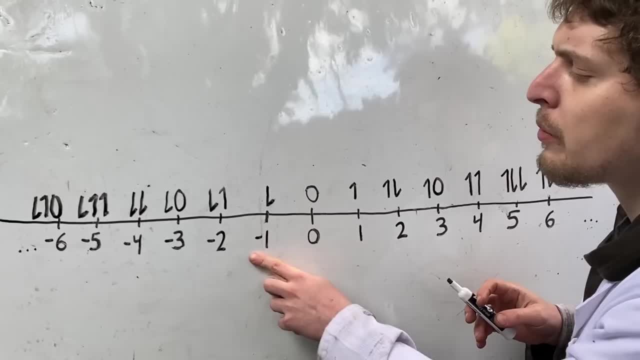 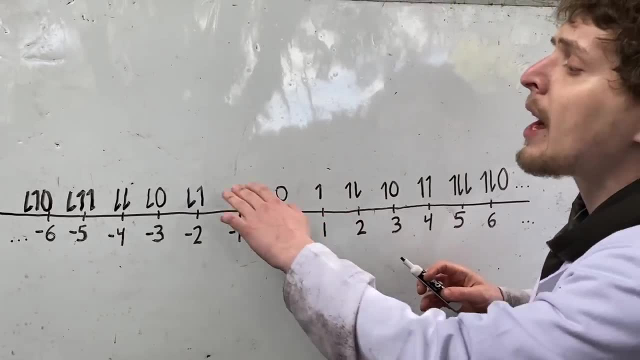 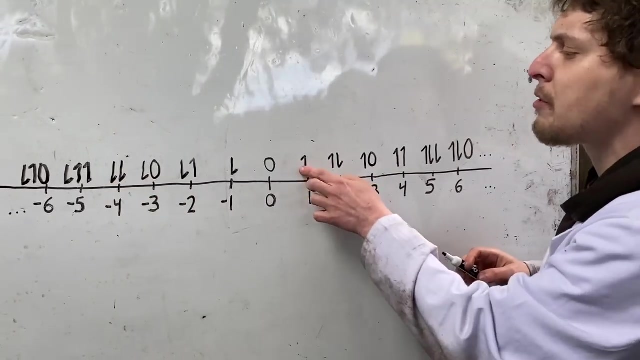 handle negative numbers. Not only can we represent the negative numbers without needing a minus sign in the representation, and we can recognize them, compared to the positive numbers, by what the largest digit is using, whether the largest digit spot in the number is a, 1 or a. 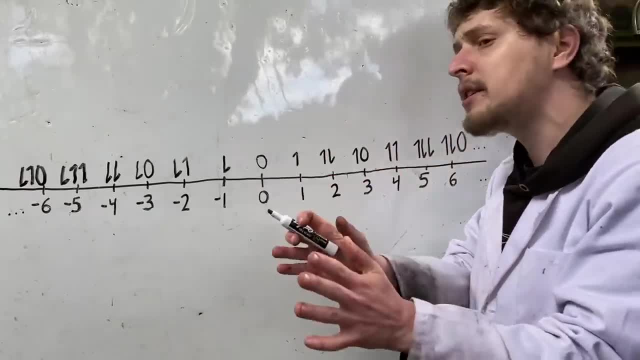 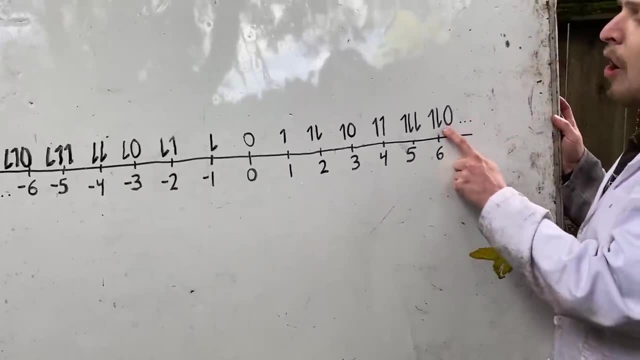 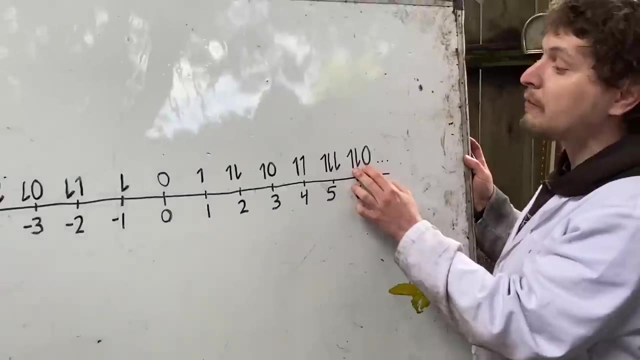 negative 1,. but also it's very easy to flip a number into its negative version or vice versa. All you have to do is take all of the non-zero aspects of that number and switch their sign the 1's to negative 1's and the negative 1's to 1's. 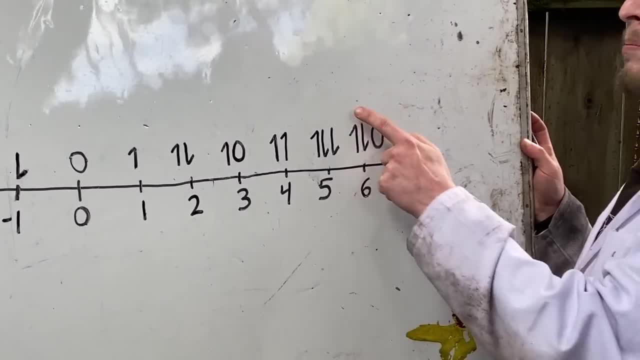 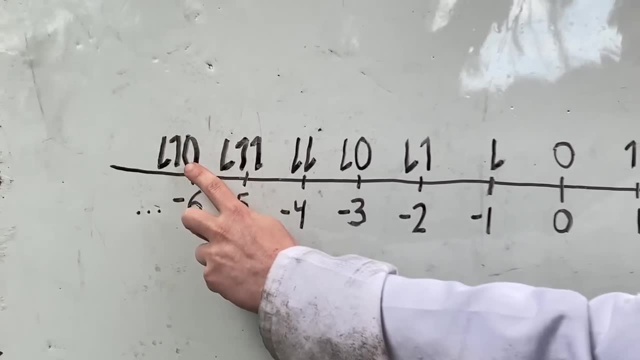 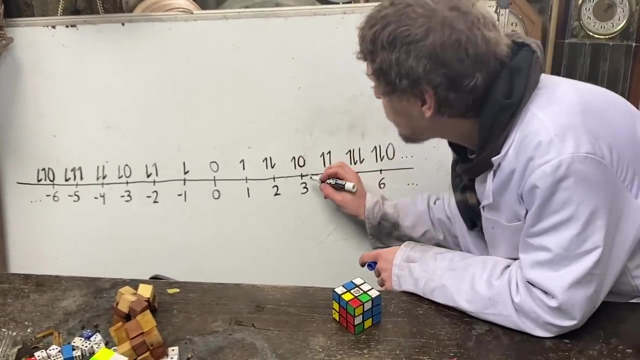 For example, with 6 here that's like up-down neutral and the flipped version of 6 is down-up neutral. Another cool trait of balanced ternary and other balanced bases is that if you zoom into a number that isn't a whole number, such as pi. 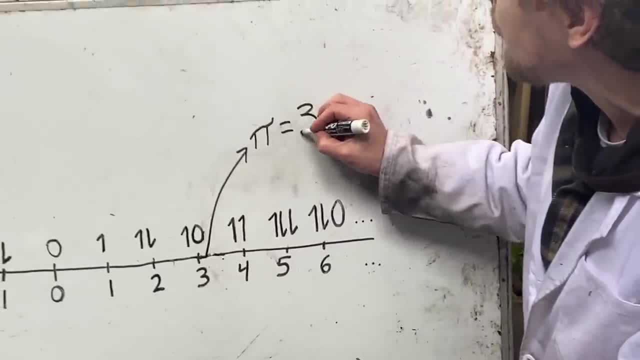 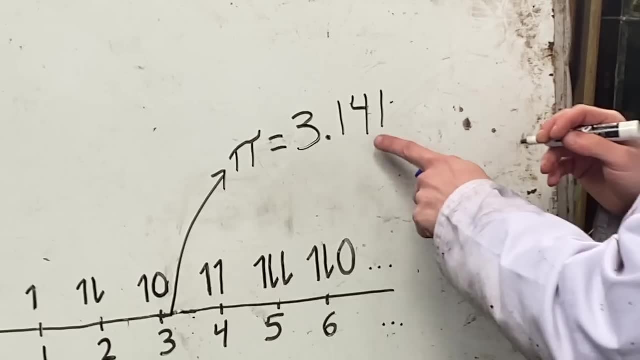 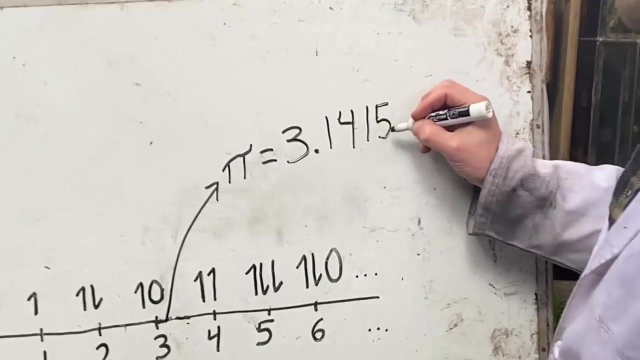 which normally we'd write the decimal form as 3.141, assuming I'm going to write more digits, Otherwise that spot would round to a 2.. But if I continue the digits, it's 1,, 5, assuming I'm going to write more digits, because otherwise that 5 would round to a 6.. 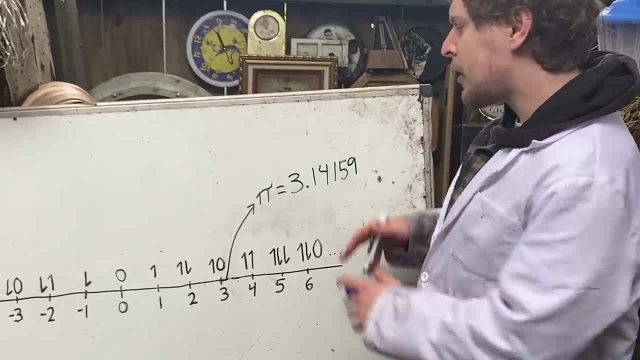 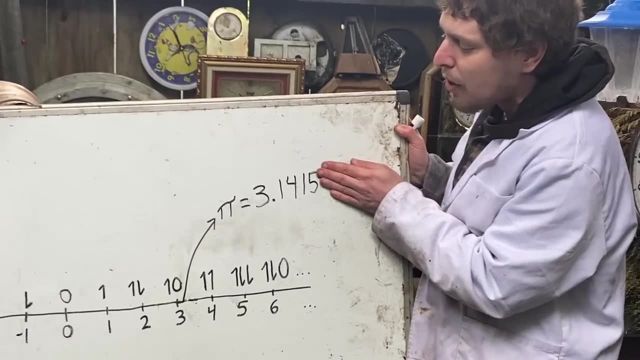 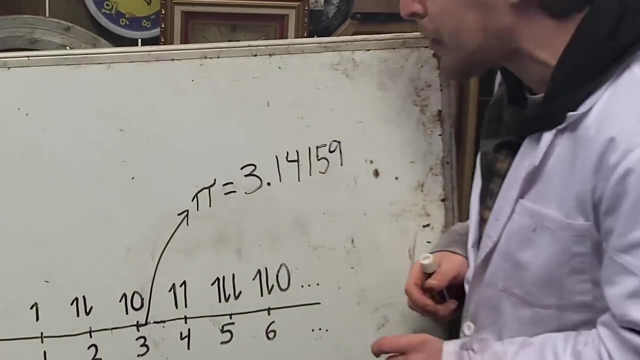 The next one is a 9. And in general in our base-10 system and similar bases, If we ever lose the end of part of a number or truncate it at a certain point, it's not always the same as the rounded form of that number. 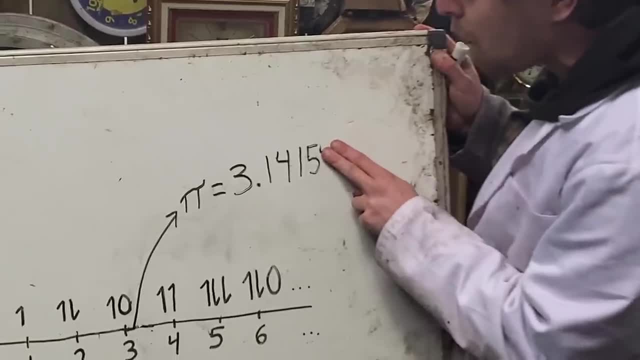 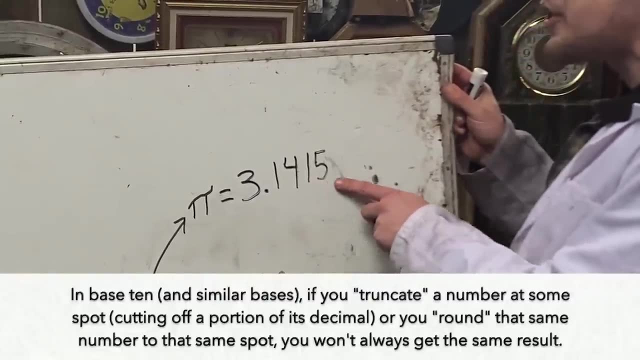 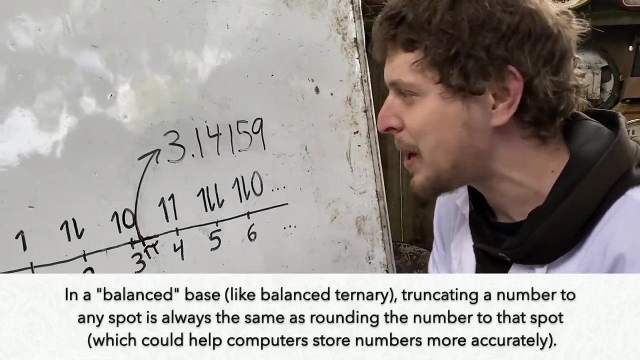 Meaning that if you were trying to write the first four digits of pi after the decimal, you have to pick between either writing the proper digit that's at that spot or writing the properly rounded form. But in a balanced base any truncation is the same as rounding. 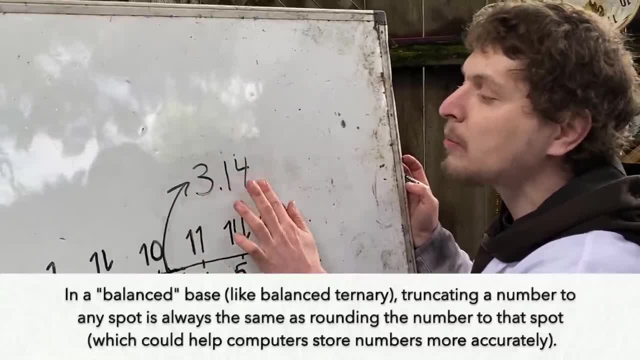 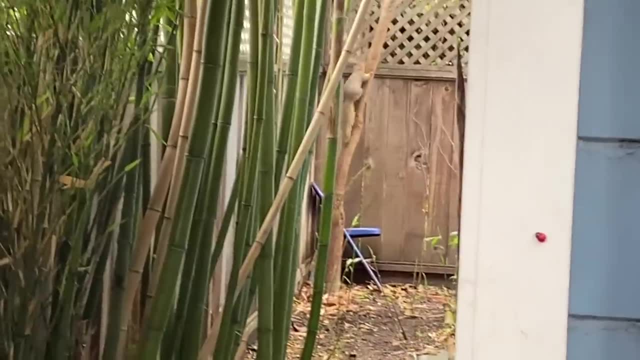 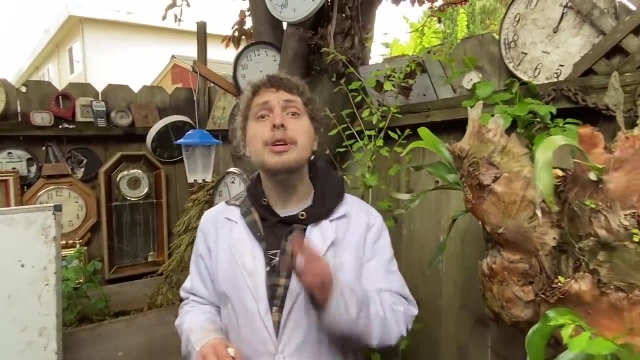 Any time you only express a smaller portion of a number like that, it's the same as if you rounded to that spot Even outside of computers. there are other ways in which balanced ternary could be useful in a society, Like if there was a currency system where coins were. worth powers of three, one, three, nine, et cetera. two people who each had one of each of those coins with them could negotiate a transaction of any amount between them. that added, slash, subtracted- sort of like the balance scale thing from earlier into one of the people having given the other any amount. 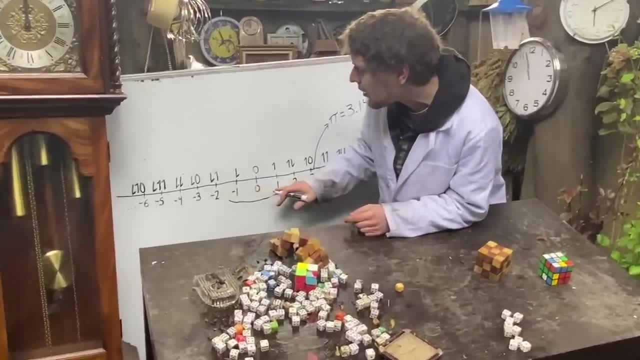 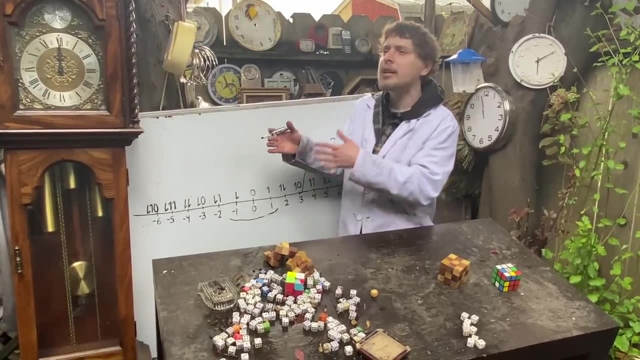 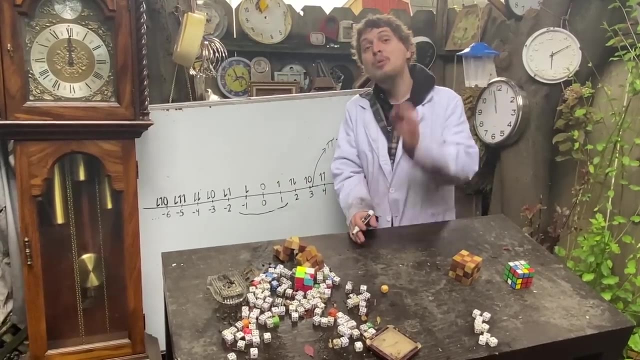 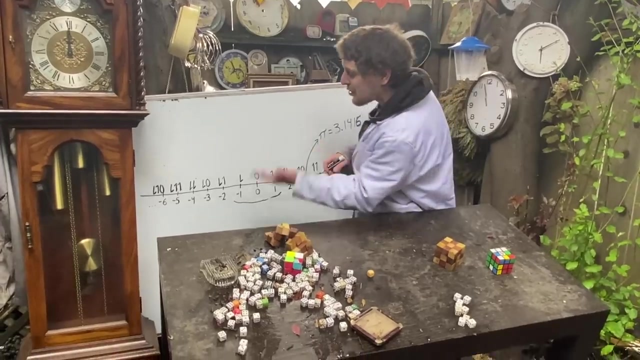 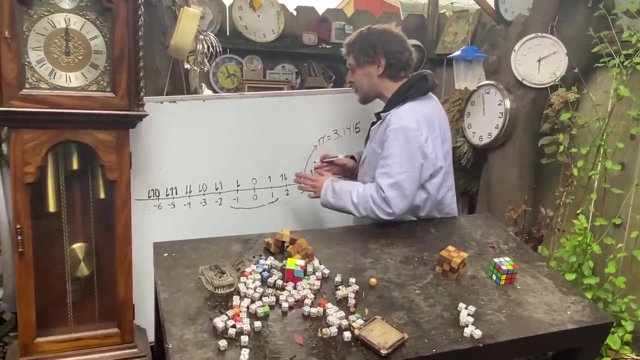 There are also some special abilities that both balanced ternary and unbalanced ternary have. They make them more efficient at storing information by certain metrics compared to either binary or larger numbered bases, And we'll return to that in an episode about what I call purely threven numbers, because those which most people call the powers of three are what the places in these numbers stand for.